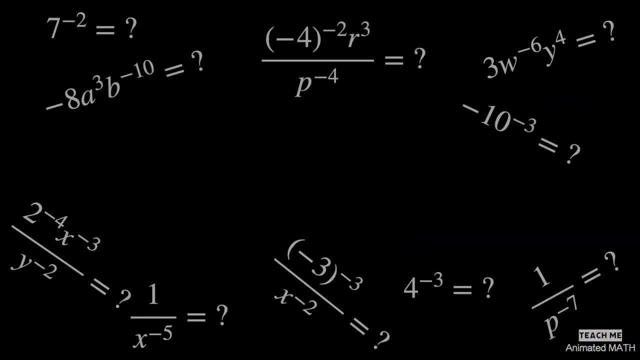 below. There will be a three-second countdown before I start solving each problem. You can pause the video and solve it on your own first, or just watch the video straight. All right, let's start solving. Rewrite the expression using the reciprocal of 7. 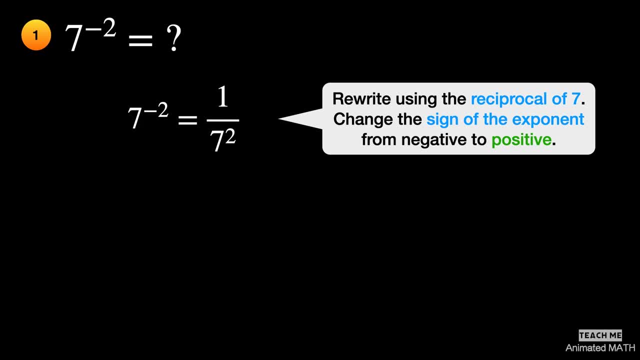 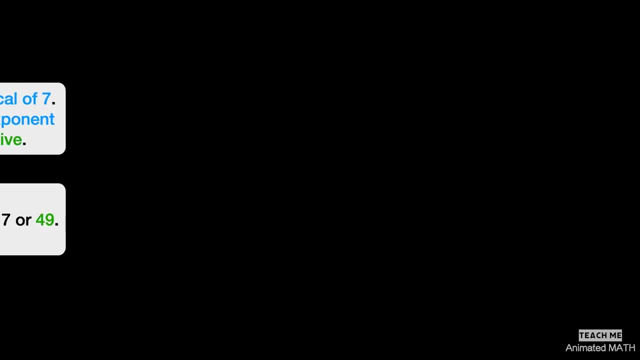 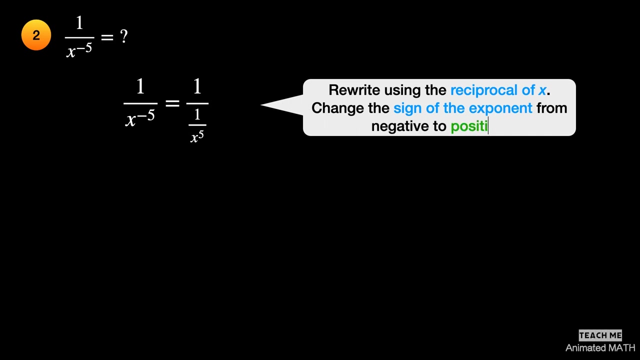 and change the exponent to positive 2. It is equal to 1 over 7 squared, or 1 over 49.. Rewrite x raised to the negative 5 as 1 over 1 over x to the fifth power, Then divide fractions. The simplified form is x to the fifth power. This is going to be a recurring. 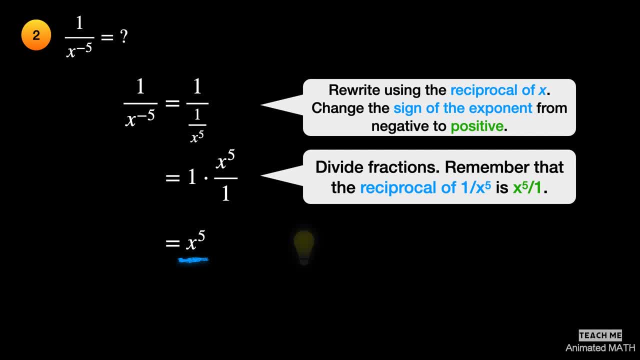 part of simplifying negative exponents. So always remember the concept that 1 over a number with negative exponent is equal to that specific number with a positive exponent. It is also true for a number with positive exponent to be equal to 1 over the number with negative exponent. 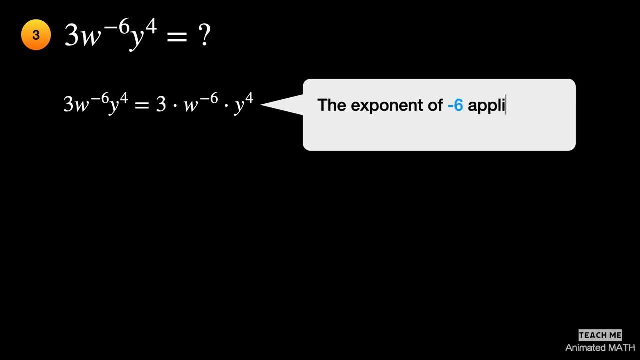 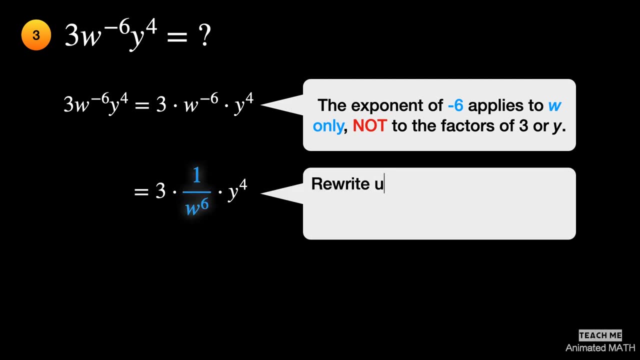 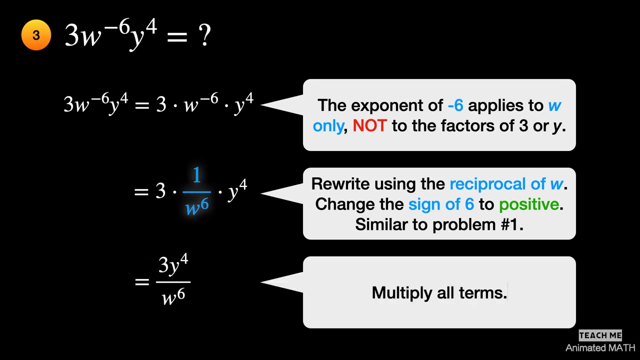 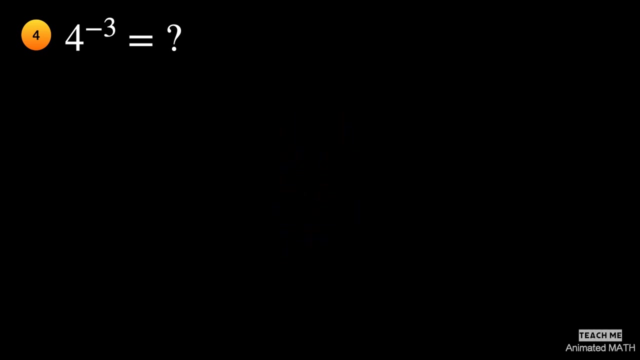 The exponent of negative 6 applies to 2 over x to the fifth power. The exponent of negative 6 appears to be the exponent of定junc semana, or single belong to x due to thekaa minus x. You can follow the Coldplay weeks in the related tutorials and watch videos from time to time. 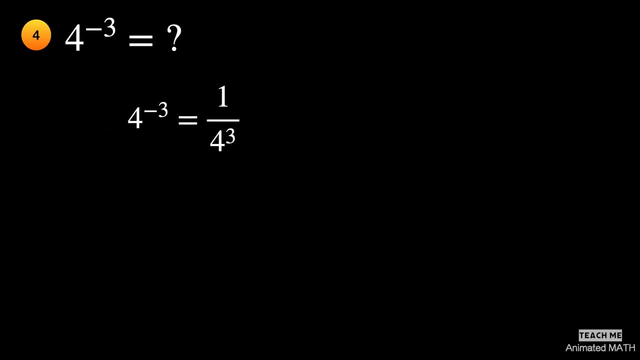 Rewrite the expression using the reciprocal of 4 and change the exponent to positive 5 or 1 over x to the sixth power. Then simply φ is equal to Emian's е, e to the fourth power, and then write W. In this içiny the same survives. W to the negative 6th power. 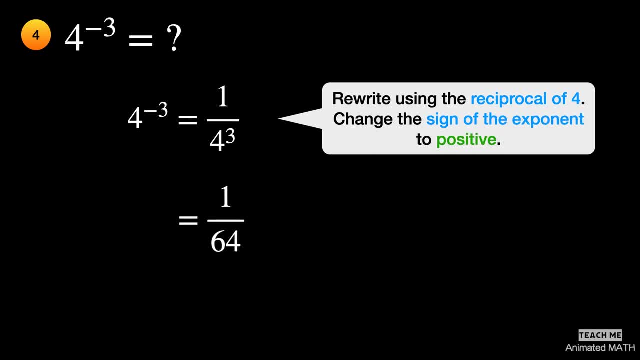 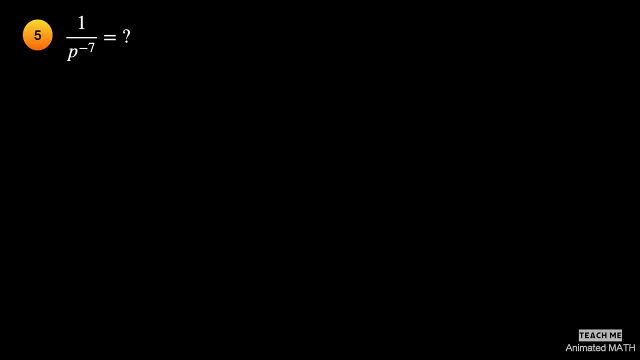 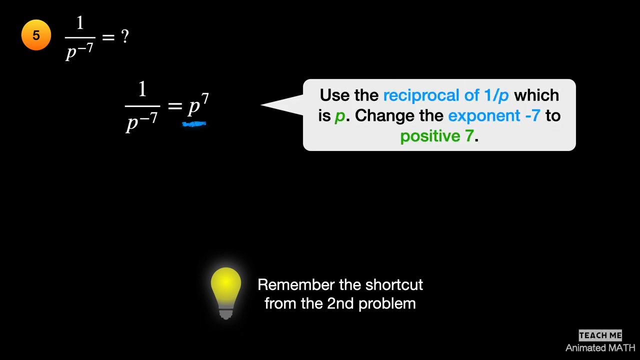 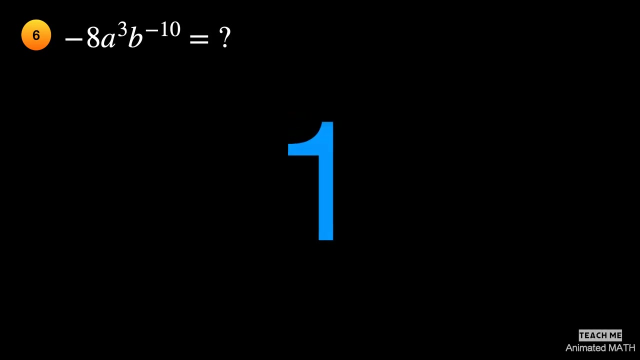 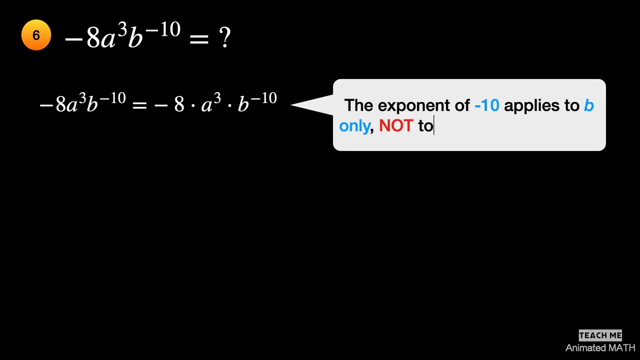 to positive 3.. It is equal to 1 over 4 cubed or 1 over 64.. Remember the shortcut we discussed in the second problem. This expression is simply equal to p to the 7th power. The exponent of negative 10 applies to b only, not to the factors of negative 8 or a. 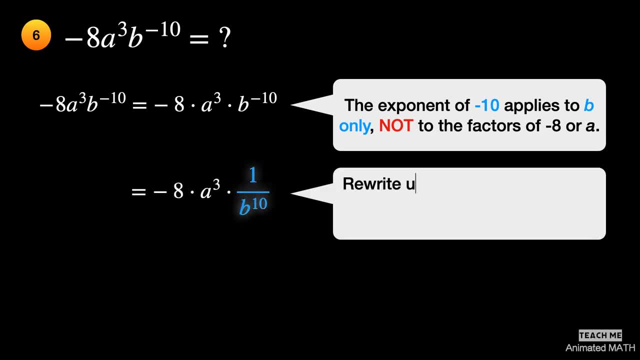 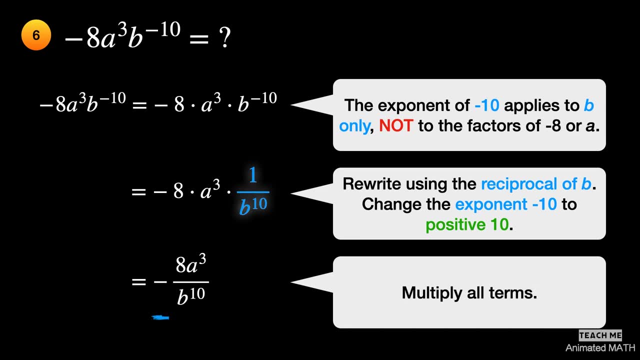 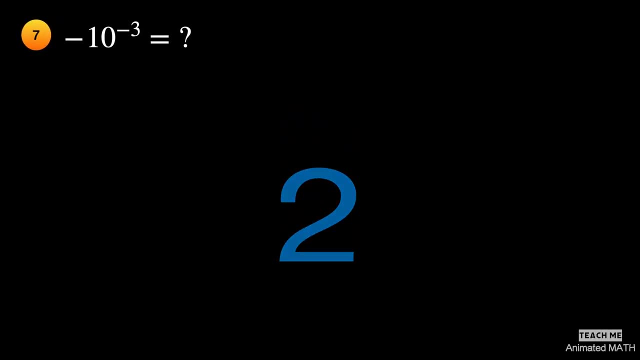 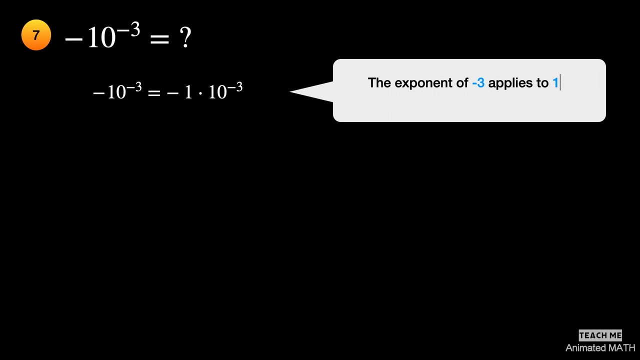 Rewrite b raised to the negative 10, to 1 over b to the 10th power. Simplifying it will show negative 88 cubed over b to the 10th power. The base for the exponent of negative 3 is 10,, not negative 10.. 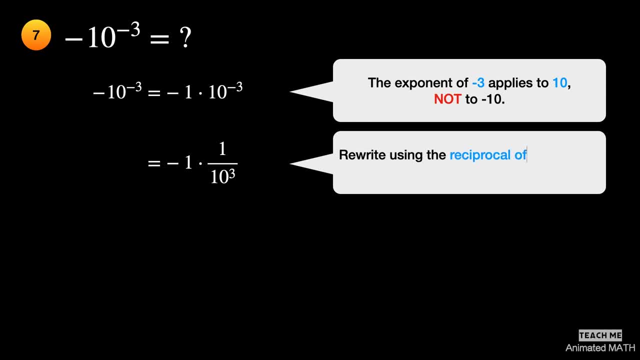 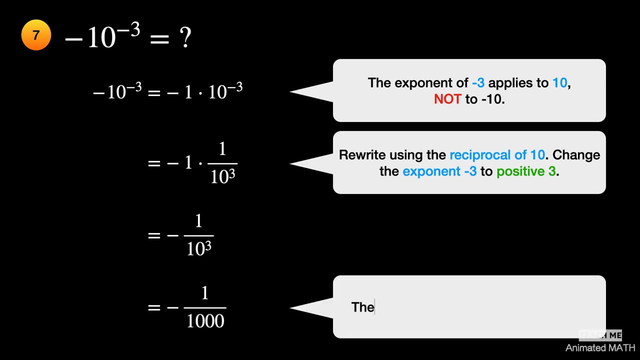 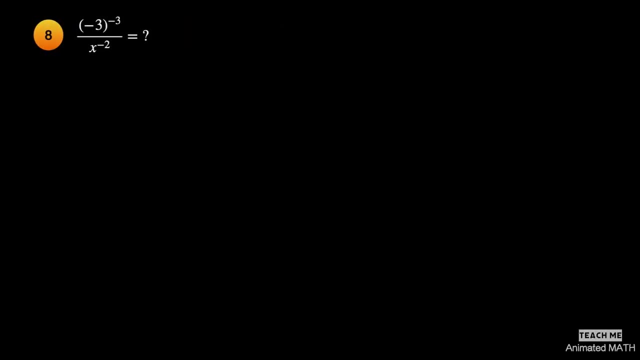 Rewrite the expression using the reciprocal of 10 and change the exponent to positive 3.. It is equal to negative 1 over 10 cubed or negative 1 over 1000.. The exponent of negative 3 applies to negative 3 only. 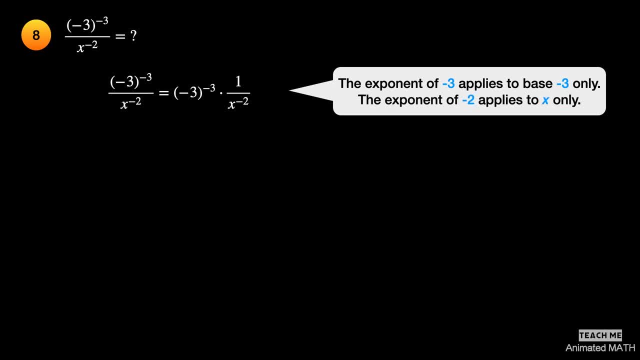 And the exponent of negative 2 applies to x only. Rewrite negative 3 to the negative 3rd power using the reciprocal of negative 3 and change the exponent to positive 3.. Simply put x in the numerator and change the exponent to positive 2.. 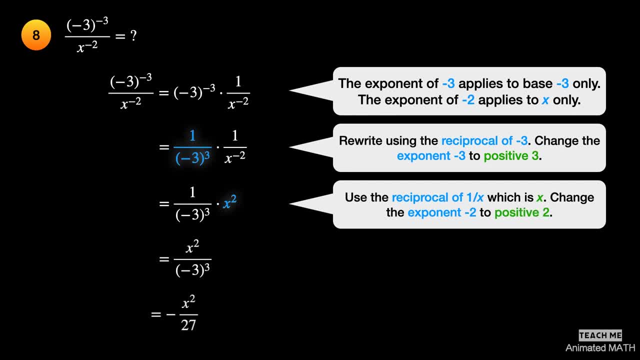 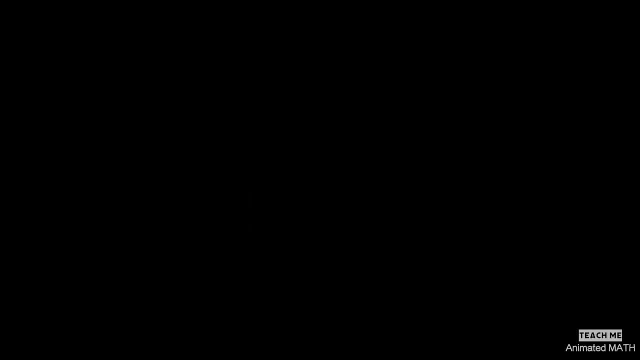 The cube of negative 3 is equal to negative 3.. The exponent of negative 3 is negative 27.. The final answer is negative x squared over 27.. The exponent of negative 4 applies to base 2 only. Negative 3 applies to x only. 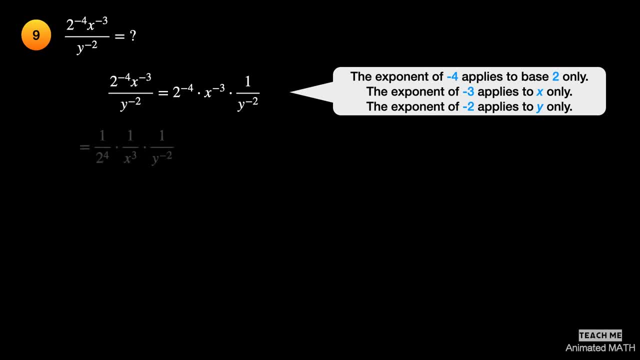 And negative 2 applies to y only. Rewrite the expression using the reciprocals of 2 and x, Then change the exponent to negative 3.. There are exponents from negative 4 and negative 3 to positive 4 and 3.. 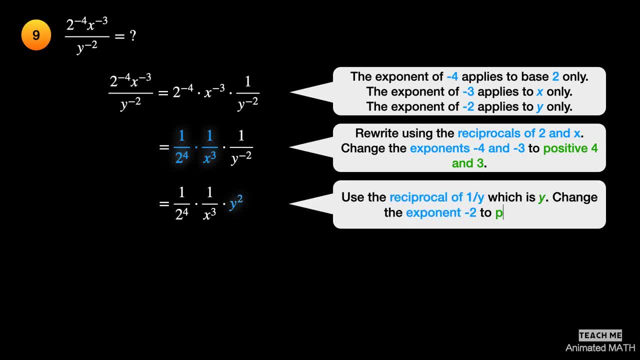 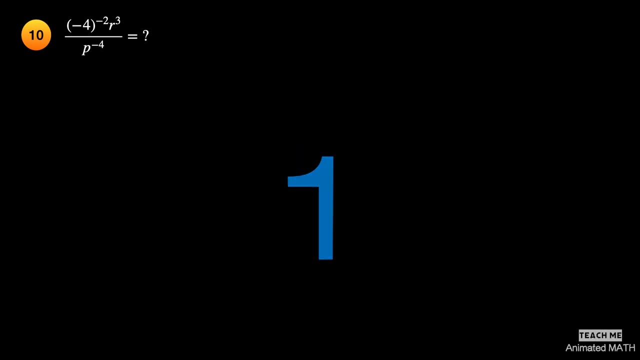 Rewrite 1 over y raised to the negative 2 to y squared. Simplifying it will show y squared over 16 x cubed. The exponent of negative 2 applies to 2.. applies to base negative 4 only and the exponent of negative 4 applies to p only.